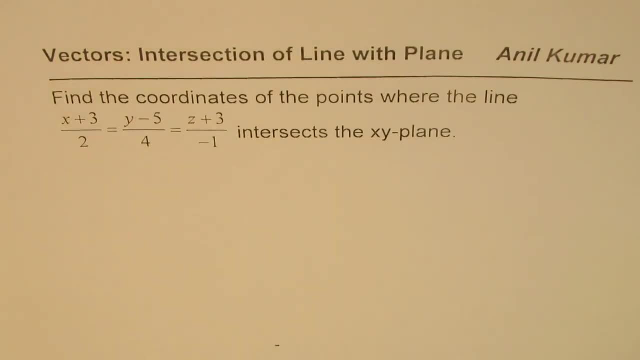 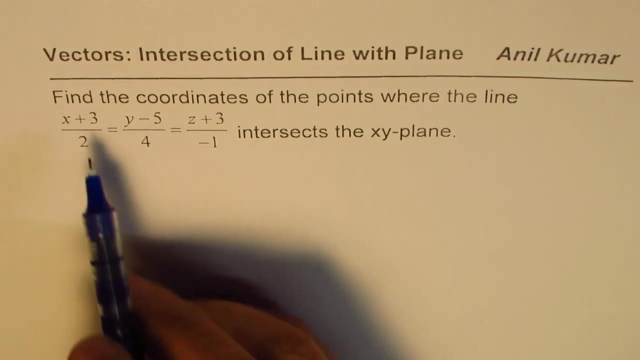 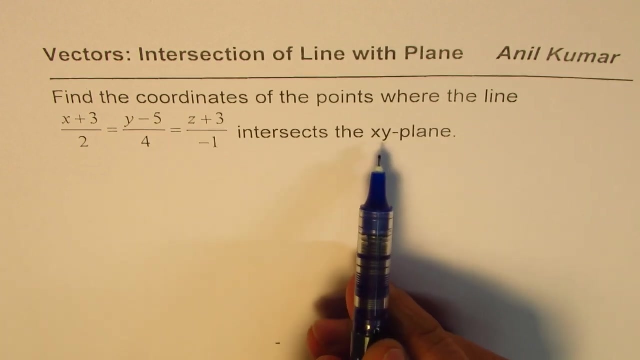 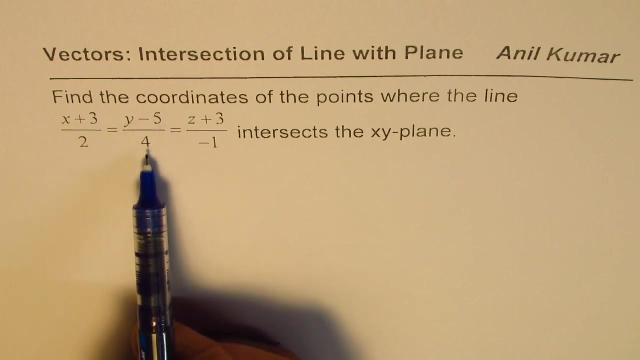 I am Anil Kumar, sharing with you a very important test question on intersection of line with plane. The equation here is: find the coordinates of the point where the line which is given in symmetric form intersects the xy plane. The equation of the line is: x plus 3 divided by 2 equals to y minus 5 over 4 equals to z plus 3 over minus 1.. 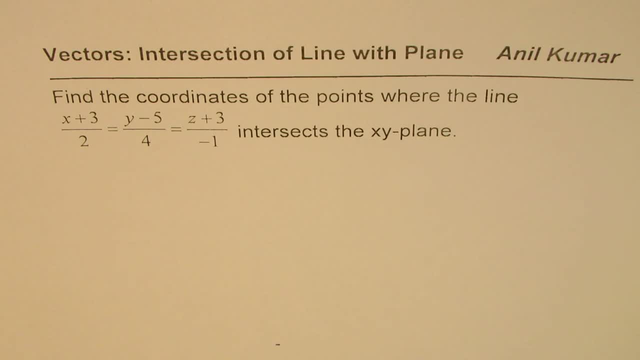 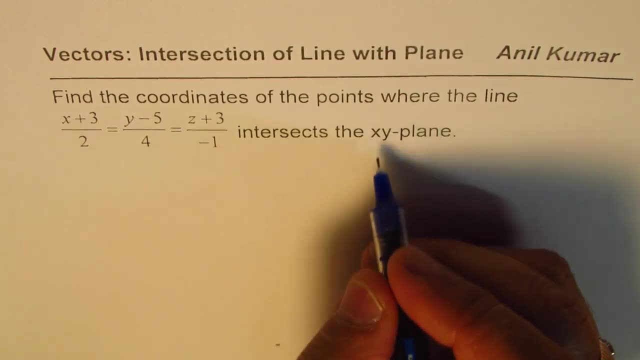 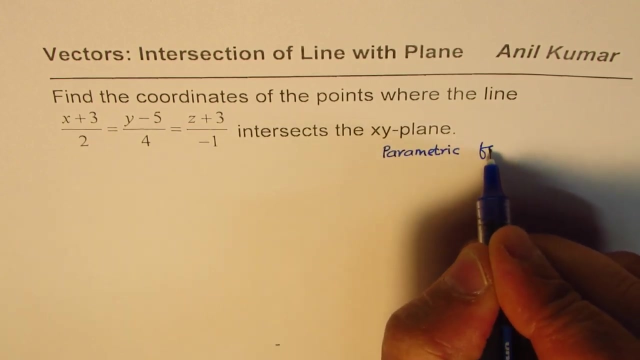 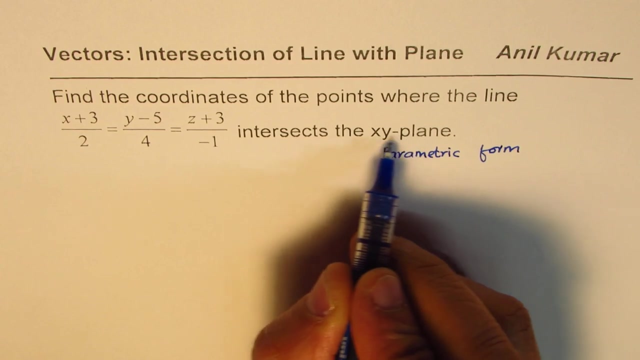 You can pause the video, answer the question and then look into my suggestions. Now, to solve such a question, we'll actually first write the parametric form of the equation right, And then we'll find the parameter by placing intersect. xy plane means what? 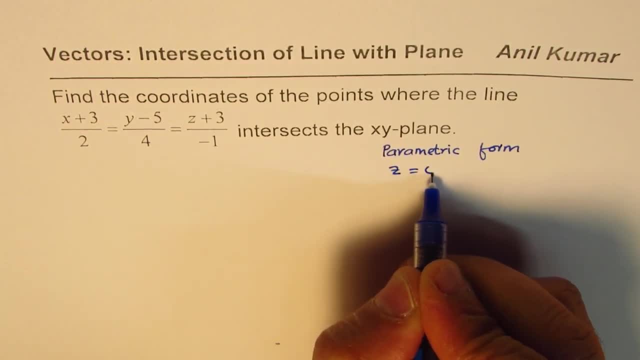 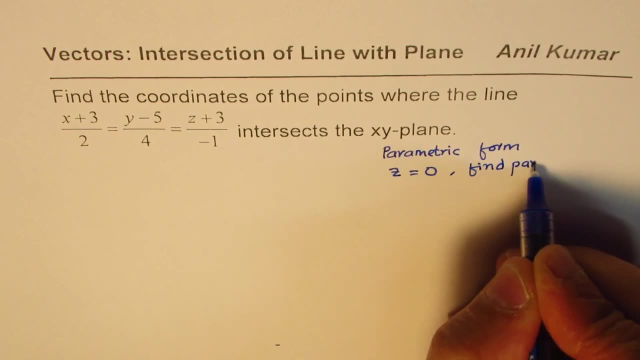 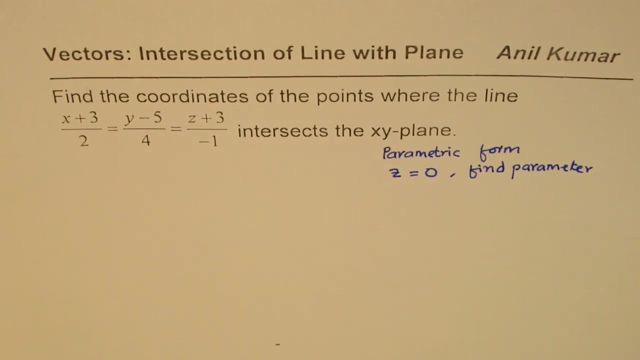 By placing z equals to 0, right. So next xy plane z value will be 0, right. Find parameter. So these are the two steps required. You can actually pause the video, answer the question and check your solution. 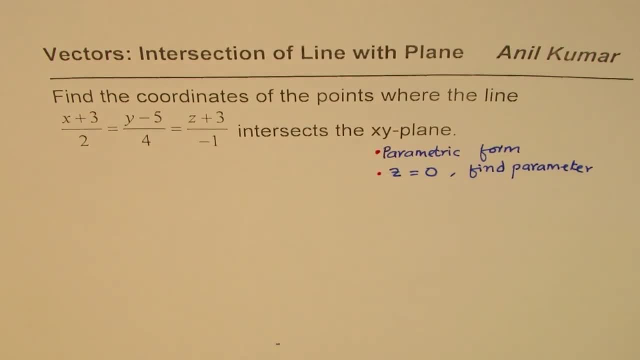 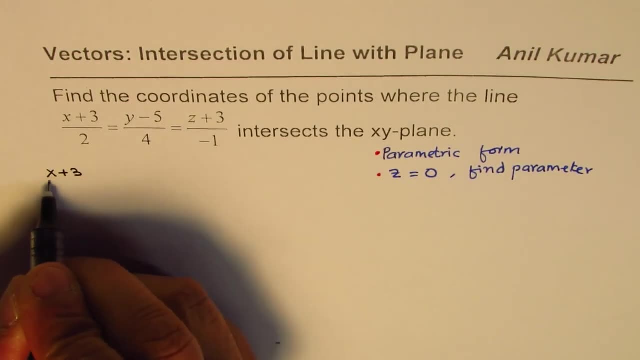 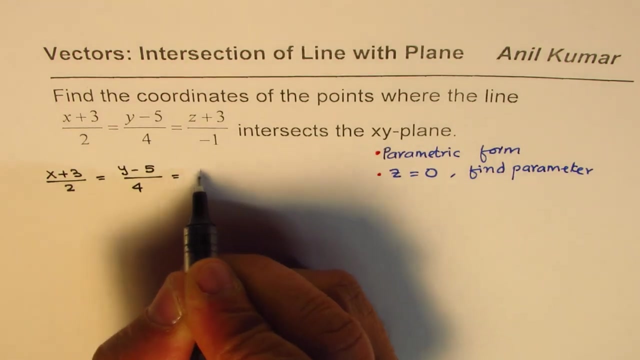 Okay, So now, first step: how to write the parametric form. Well, the equation given to us is: x plus 3 over 2 equals to y minus 5.. So we can write the parametric form of: x plus 3 over 2 equals to y minus 5 over 4, equals to z plus 3 over minus 1.. 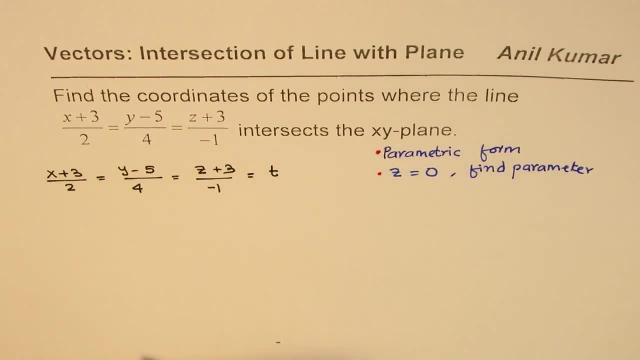 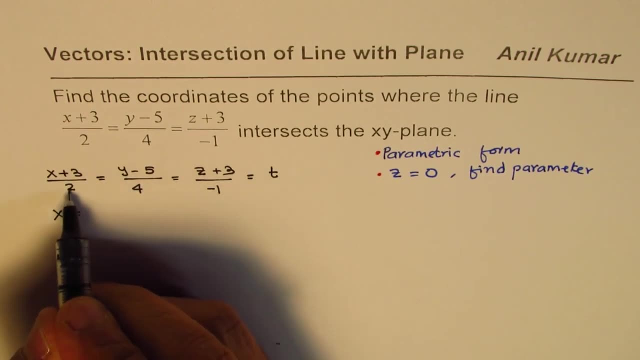 So all this will be equal to the parameter. let us say t. Now, one by one, we can write parametric form. starting with the first one, x equals 2.. 2 times t. right, Let me write 2 times t first, and then minus 3, okay. 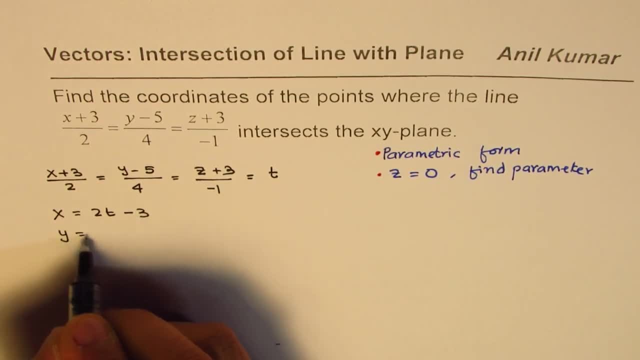 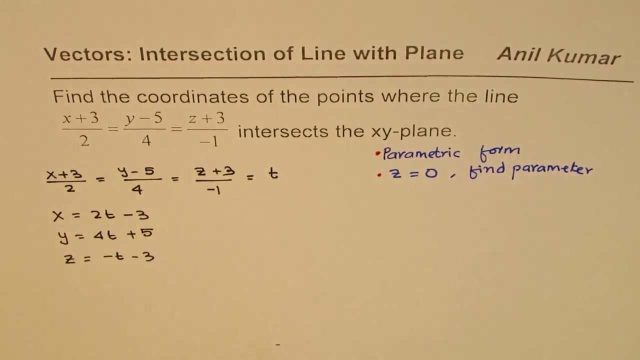 The second equation: y equals 2. 4 times t Plus 5. And z equals to minus t minus 3, right, So we get three different equations. Now from these three equations we have to get x, y, z coordinates where the line intersects x, y, plane, right. 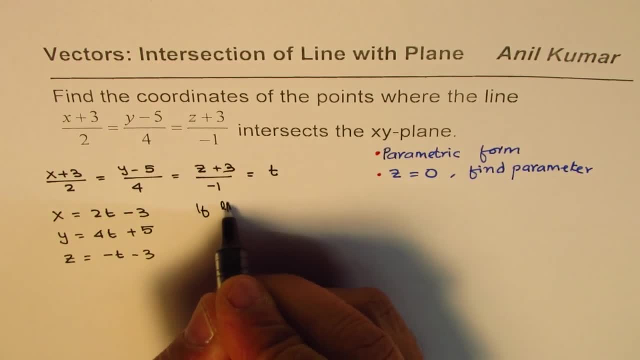 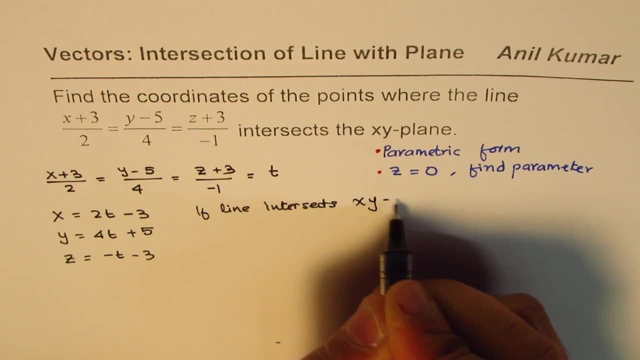 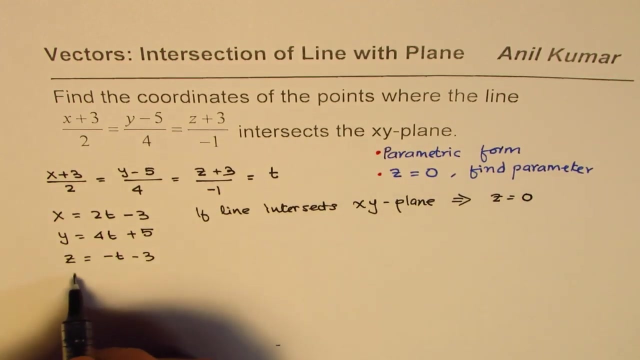 So if line intersects x, y plane, that implies that z should be equal to 0, right? So if I equate z equals to 0, I can find the value of t, So minus t plus 3.. 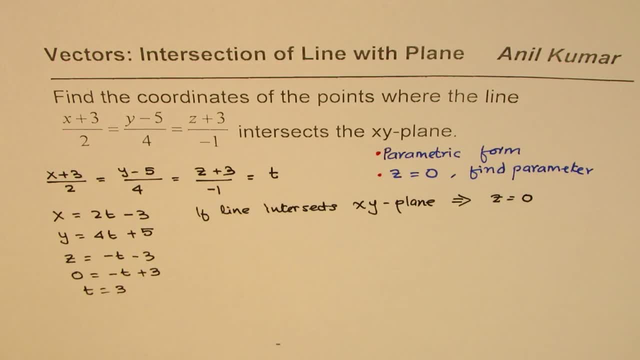 So bringing this t equals to 3, right? So that gives us the value of t. So we'll call this as our equation 1.. So we know what t is. Once we know what t is. Once we know what t is, we can find x and y coordinates, right? 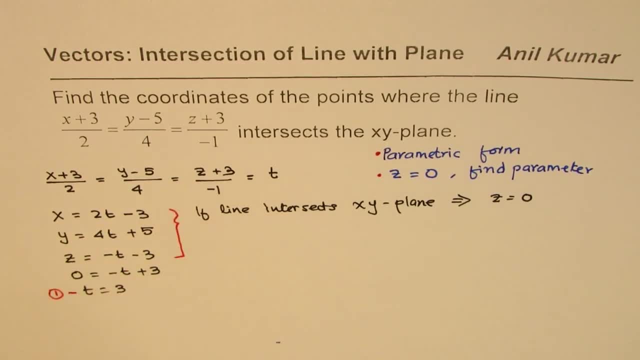 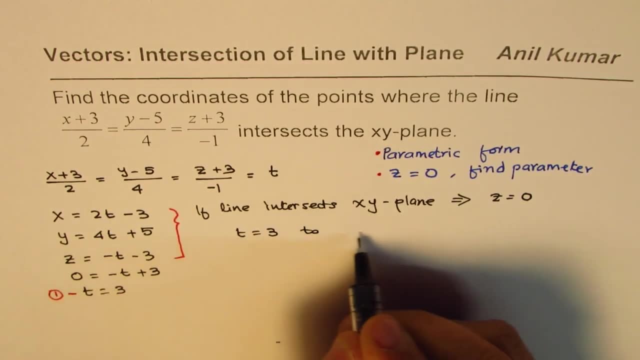 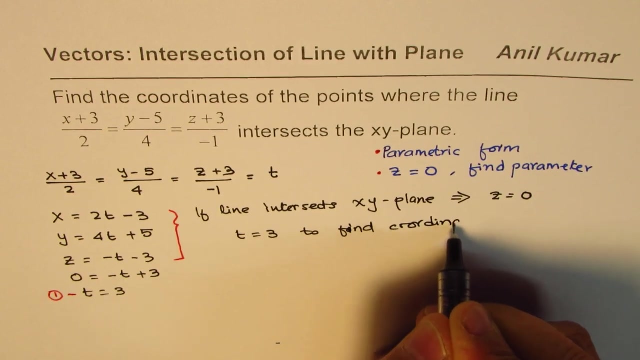 So we'll substitute. So that's our parametric equation. So in this equation we'll substitute t equals to 3 to find coordinates. I hope the steps are absolutely clear. So x coordinate will be what x will be. t is 3.. 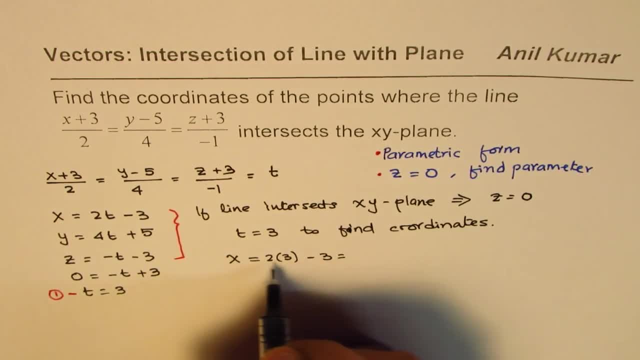 So 2 times 3.. 3 minus 3,, which is 6 minus 3, is 3.. y value will be equals to 4 times 3 plus 5,, which is 12 plus 5, is 17.. 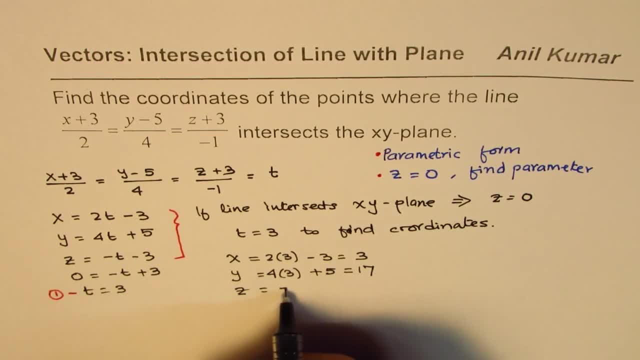 And z, we know should be 0. But let's confirm right, Minus 3 plus 3, that is 0. So it intersects x- y plane at a point. Let's call this point as P. 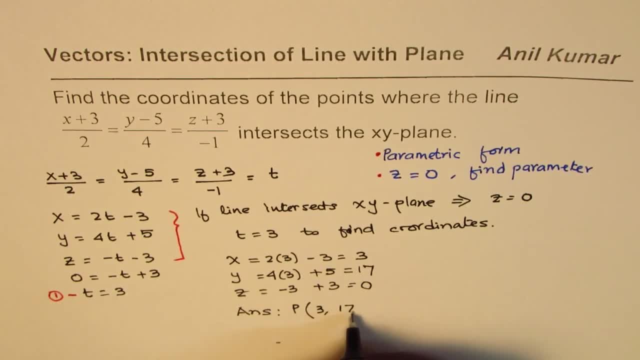 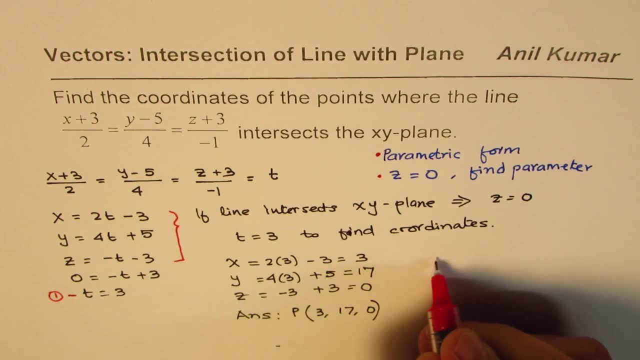 Which is going to be 3, 17,, 0.. Correct, So that is how we can answer this question. Now, as an added exercise, the question for you is to find intersection with y z plane and x z plane, right. 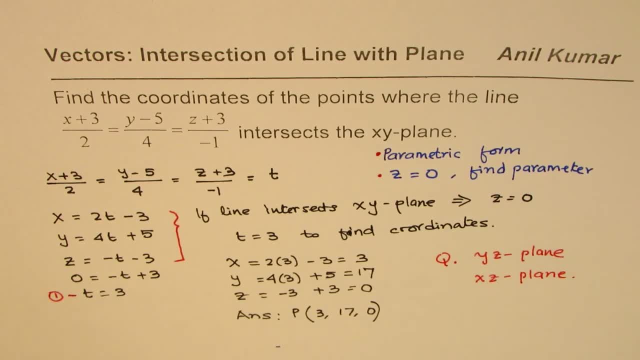 So let that be practice question for you to do. I'm Manil Kumar and I hope that helps. Thank you and all the best.